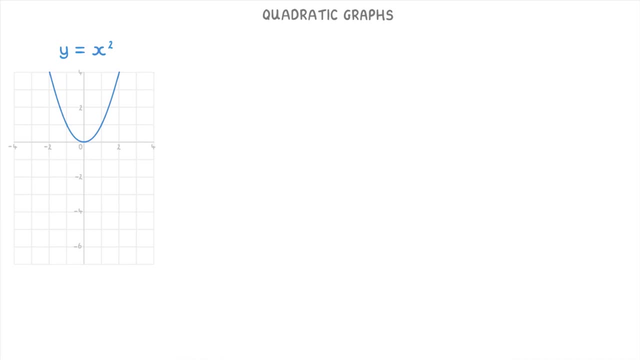 The next thing to know is that the x squared term is negative. When you only have x squared and there aren't any x terms and number terms, then the only place that your graph will cross the axis is at 0, 0.. The same goes for y equals minus. 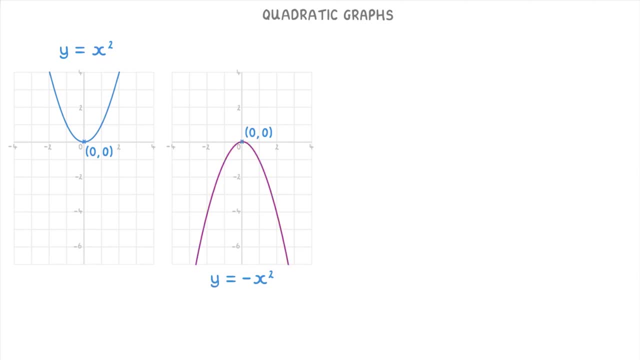 x squared, But this time it curves downwards instead, because the x squared term is negative. The more you change the equation, though, the more different the curve will look. For example, if, instead of y equals x squared, y equals y squared, then y equals y squared, y equals. 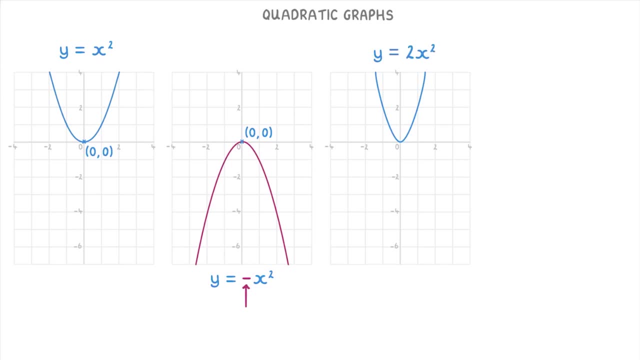 equals x squared, we had y equals 2x squared, the curve would become a bit narrower, like this: While if we had 2x squared minus 3, then the curve would move down a bit. And if we had 2x squared, 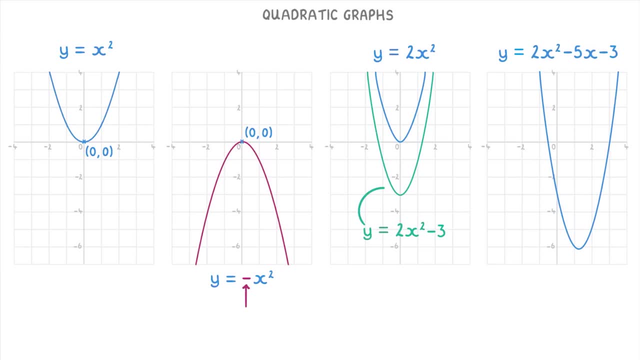 minus 5x, minus 3, that would move even further down and over to the right. You don't need to worry about how all of this works exactly and what changing each of these numbers would do, but you just need to understand that changing the numbers in the equation 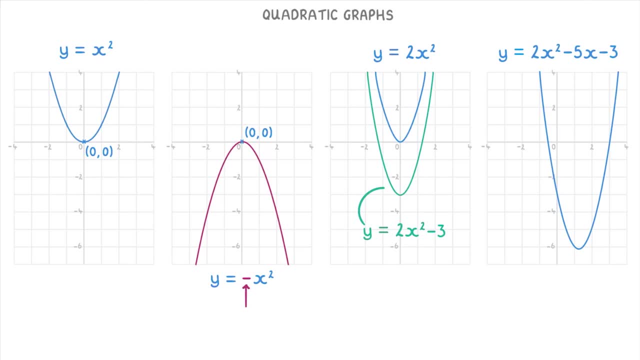 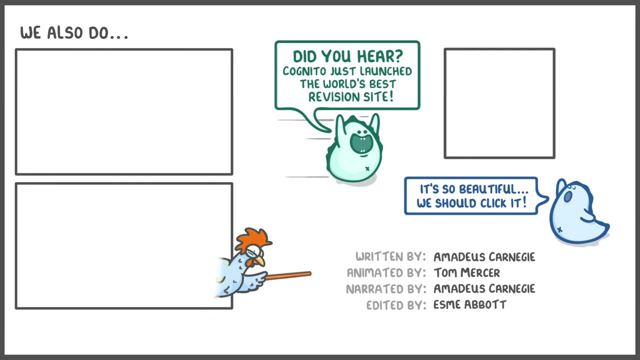 will change the shape of the graph. Anyway, that's it for this video. it was only a quick one today, So cheers for watching and we'll see you next time.